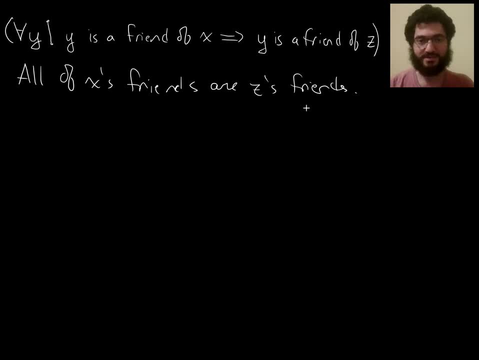 up here by some other dummy variable and it would not change the meaning. So in this proposition, which could be written in either of those ways, we would say: well, if you write it the first way or the second way, we would say x and z are free variables here. 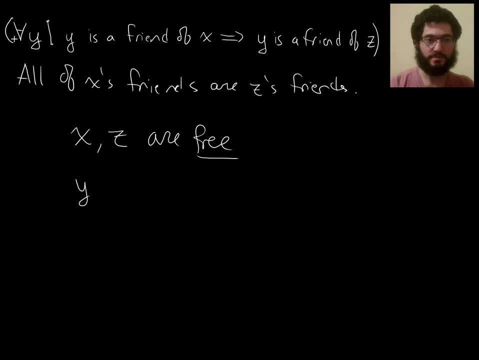 They are not bound, Whereas we would say y, especially if you write it the first way where you can see the y showing up but it's not really there. you would say the y is a bound variable. So what is in the symbolic formalism? what's doing the binding? 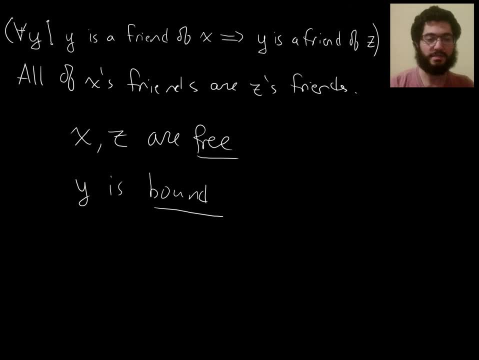 what tells us for sure that y is a bound variable is this fact that y is quantified by the for all. Now there are other ways for a variable to be bound: It could be quantified by there exists, or there's a third way which we will learn about soon. today, 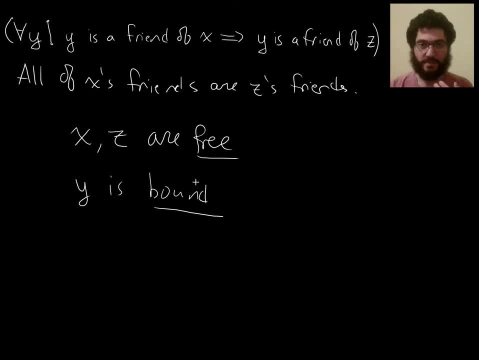 So this is the general idea that, in terms of meaning, when a variable is bound, that means it's not really there. You can see with the second way of writing the sentence: there are no y's, It's not really there. So if we just look at this example here: 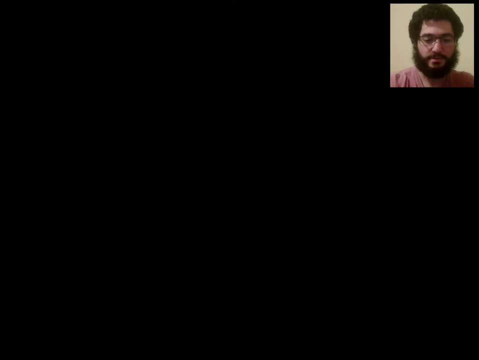 let's just look at one more example here. Okay, so I've slightly modified the example. It still looks like it involves x, y and z, If you just, you know, look at the markings, and now it says for all y if y is a friend of x. 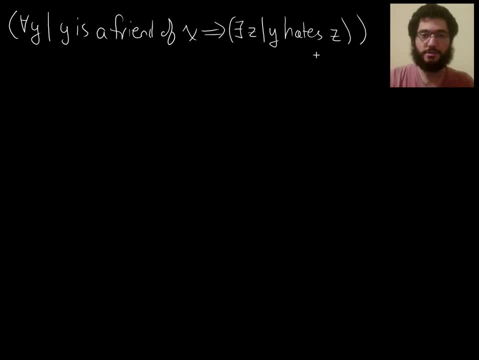 then there exists a z such that y hates z. So if I were to just write this part in plain english, it says y hates something. And if I write the answer here, the entire thing in plain english, it says: all of x's friends, uh hate something. 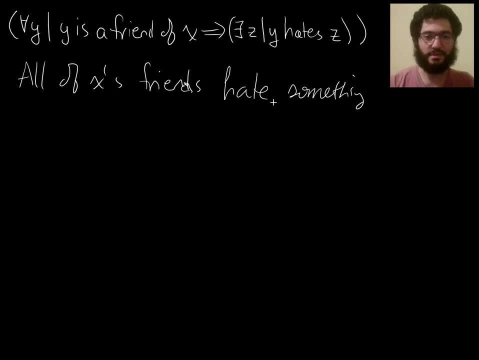 now that's kind of ambiguous. it's not clear whether it's saying there's this one thing, that all of x's friends hate that one thing, or if each of x's friends has at least one thing that they hate, but they could be hating different things. it's actually the second one, so maybe to